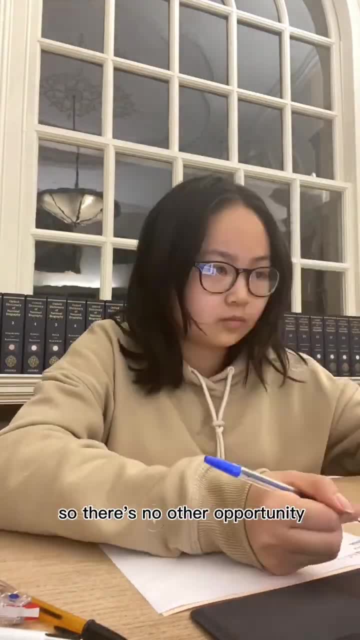 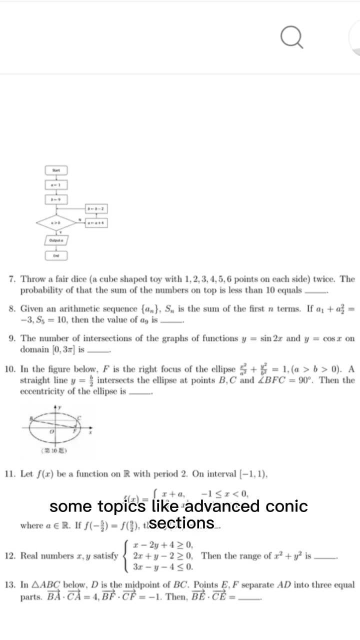 that determines which university you go to. So there's no other opportunity Now. looking at the maths component, firstly it's easy to tell that there are lots of very advanced topics on here. Some topics like advanced conic sections I definitely not seen until first year of university. 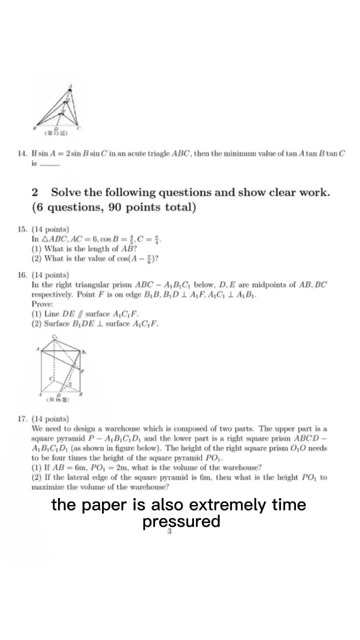 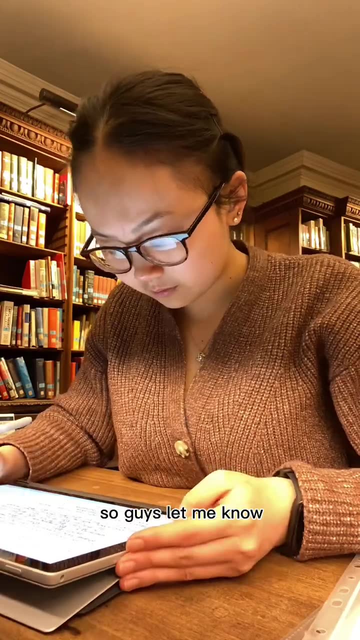 and also some statistics. The paper is also extremely time-precious, so, even though there are some easier questions on there, the hard questions took me a long time to do. So, guys, let me know, do you think this is harder? or the GEE? I'll link the GEE video down below and make sure to subscribe, Subscribe and follow along for more hard maths. 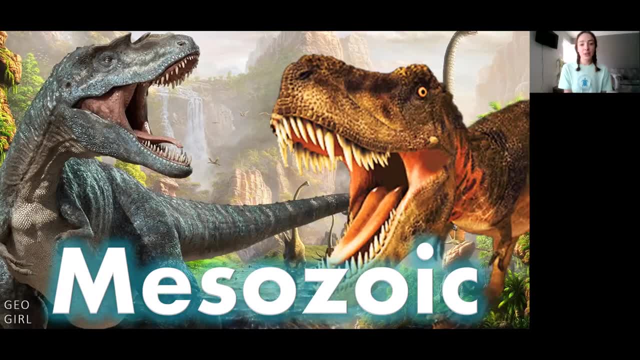 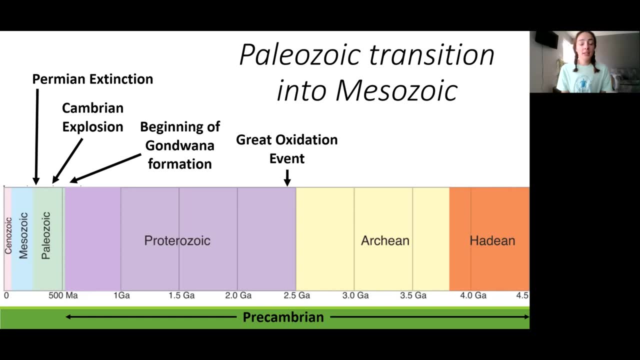 Hi everyone. today we're going to be going over the Mesozoic era, So to start I just want to review kind of what we already covered. We talked in the last two videos about the Precambrian and the Paleozoic respectively, and now we're going to move on to the Mesozoic. So down here. 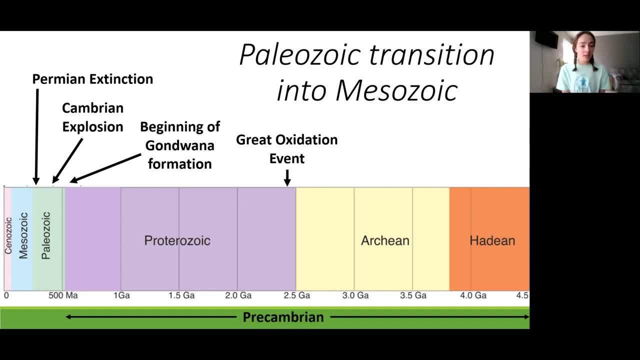 on this time scale, we can see from right to left, going older to younger, We have the Precambrian, which includes the Hadean, Archean, Perterozoic, and then we have the Paleozoic, which is the tiny green band, and then we have the Mesozoic, and this is what we're going to talk about today. 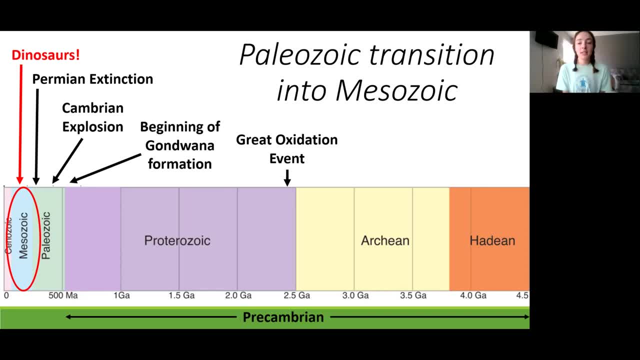 And the main event that I put on here for the Mesozoic says dinosaurs, because that's pretty much what everybody thinks about when they think about the Mesozoic, because it includes the Jurassic period, but it's a lot more than dinosaurs and so, even if you only know about the Mesozoic, 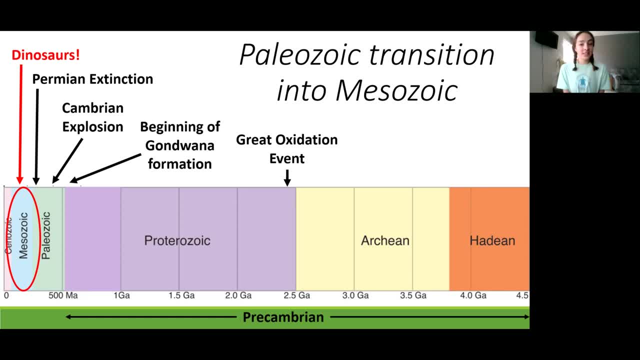 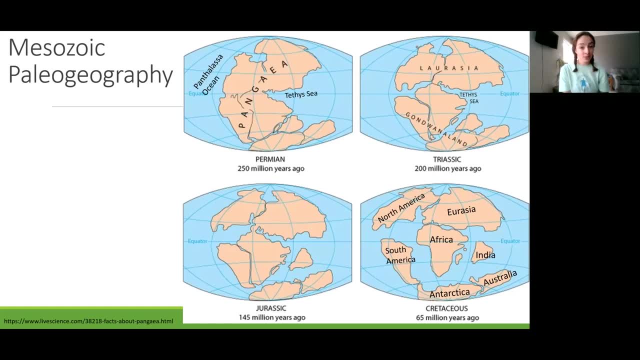 because of the dinosaurs. today you're going to learn a lot more about the events that occurred in the Mesozoic. First, I'm going to go over geologic events that occurred in the Mesozoic, so tectonic settings and paleogeography.